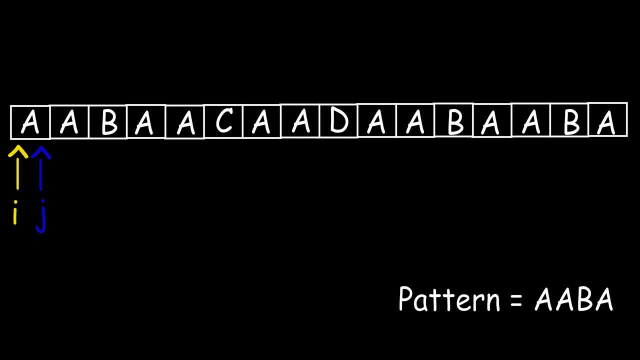 strings pointer, that is, i starts at the start of the string, that is, at index zero and j starts at i. now the pointers are at their places. now the operation begins. i is at zero, welcome, welcome, and j is at i. j starts to check if the current element is equal to the pattern's first element. 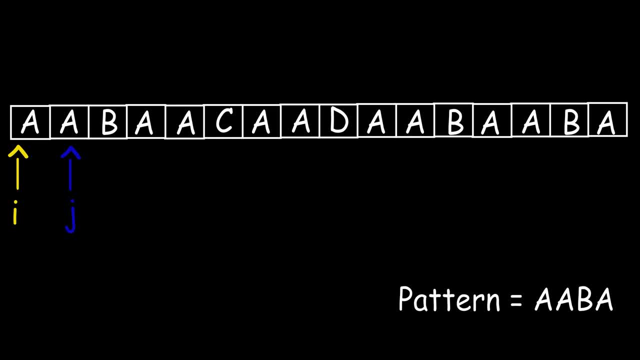 In this case it is yes. It moves to the next element. Now again, it checks for the pattern's second element. Yes, it matches The j pointer. moves to the next element. Now it checks whether the current element is equal to the pattern's third element: Yes. moves to the next element. 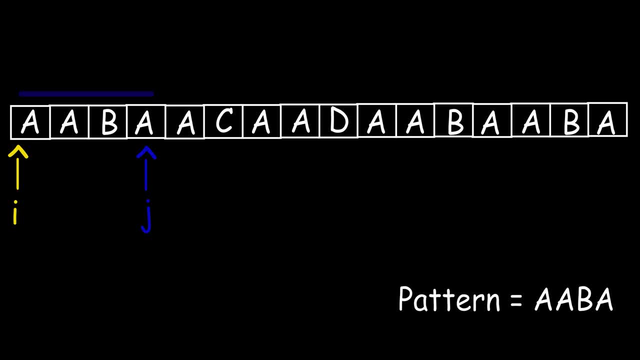 and the current element is equal to the pattern's fourth element. And yes, the pattern is found. Now let's print out the index at which the pattern is found. Now i moves one step further, as j is equal to 1.. j checks if the current element is equal to the pattern's first element. 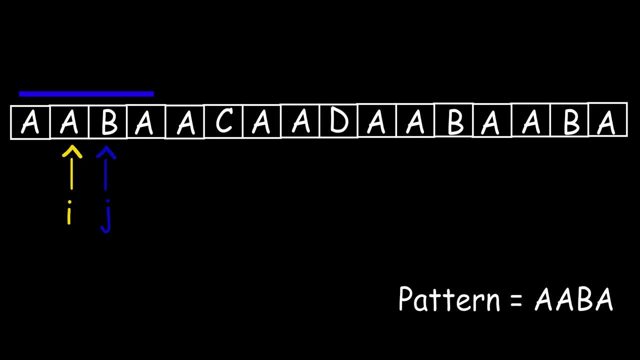 Yes, it matches. j moves one step further. Now it checks whether the current element is equal to the pattern's second element. No, it does not match. j pointer starts to stops and i moves one step further. This process continues until the end of the string Note. 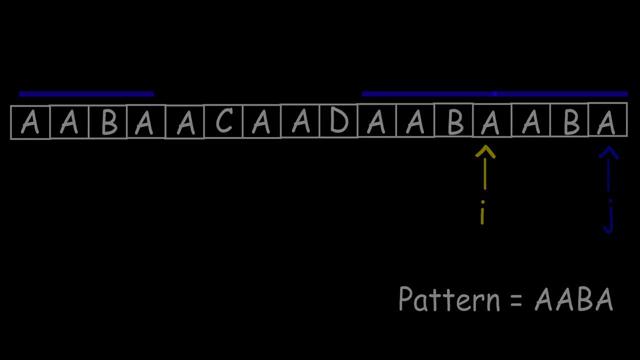 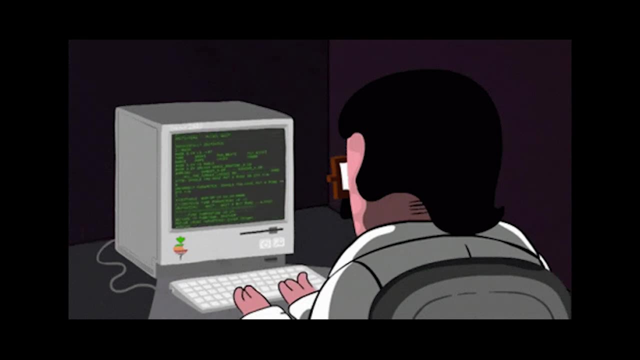 that j only moves 4 positions, ie the size of the pattern. Try to code it yourself and if you find any difficulties, you can see my code. Now let's look at the code. You have a basic structure of a C file. We have the header. 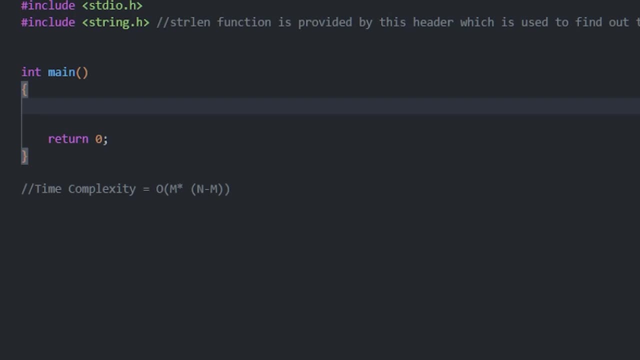 file. We have also included a stringh header file which gives us the strLength function which is used to find the length of the string. We have the main function. In the main function we have declared that text which contains the string or the main text from which the pattern have to be found. 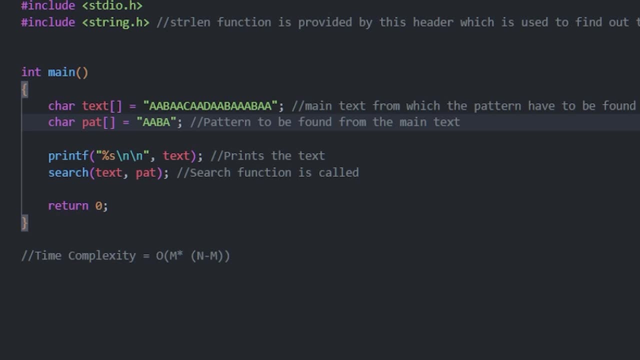 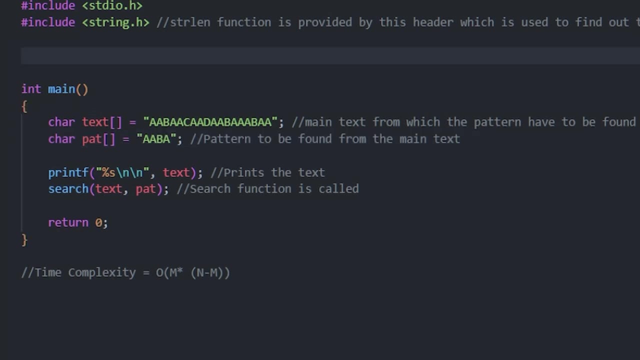 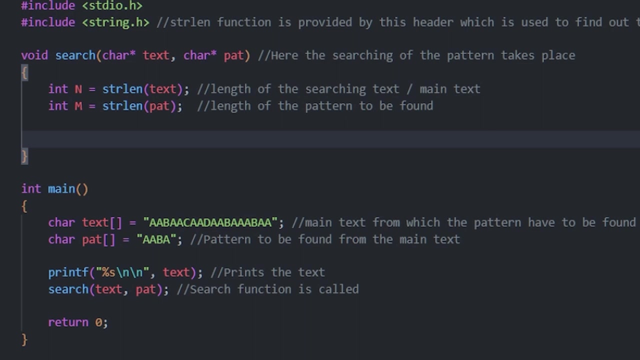 We have the pattern, that is aaba. We print the text to compare it with the index. we find out after the search is called. Now the search is called, The search function takes the parameters text and the pattern to be found. We create two variables: n and m. n contains the size.